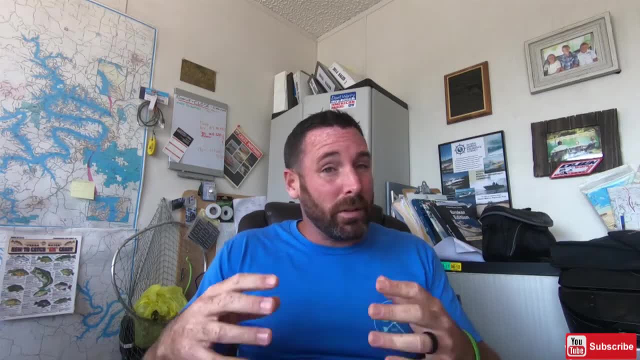 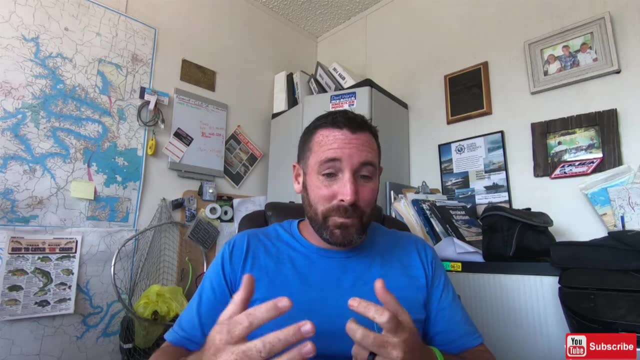 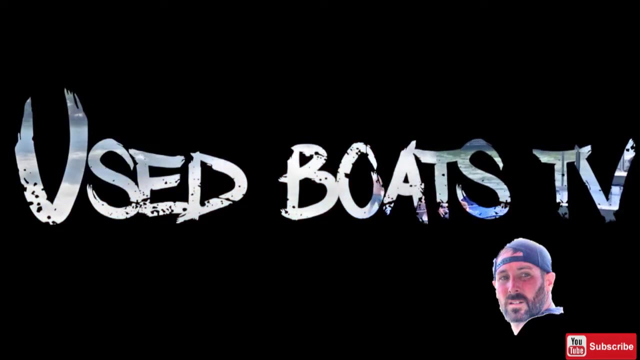 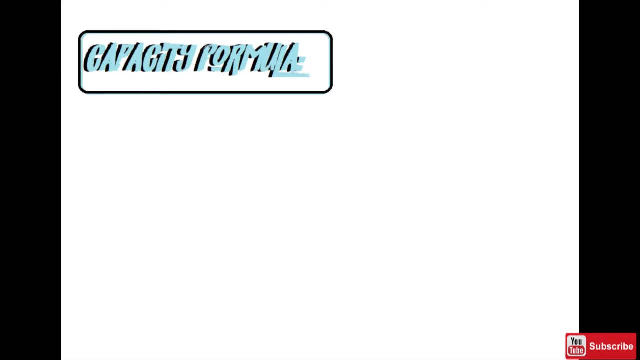 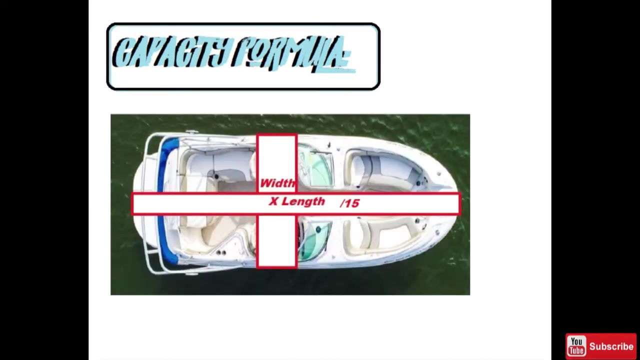 the middle of the screen. the purpose of this channel is to provide boaters and boat sales. you are with more information to help enhance your ownership or selling experience. okay, let's get on it. the math used for a capacity rating formula is pretty simple actually: length multiplied by width, divided by 15.. this will tell you just how many 150 pound people 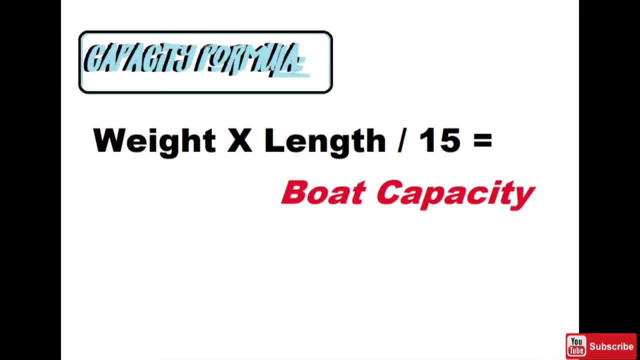 can be in the boat, or how many 150 pound people the boat will be rated for. i don't know about you, but i've got a lot more friends that weigh well over 150 than under anyways. however, the issue here is the term length isn't defined well enough, which creates a 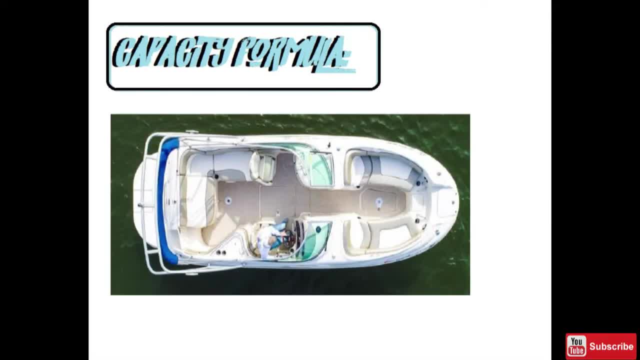 confusing issue for many boaters see. some companies use length including the swim platform, so what i would call the overall length. others use just the length of the boat by itself, without a a swim platform, while the remainder, which would be the only other way to do it, err on the side. 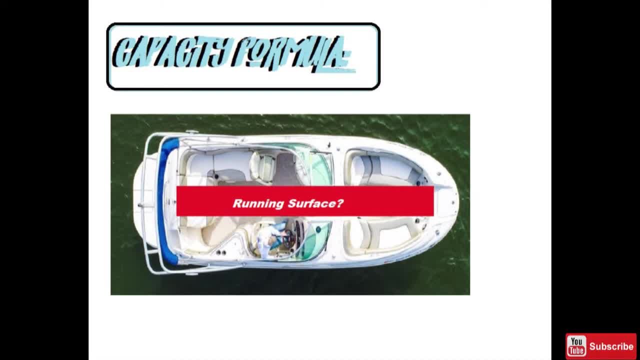 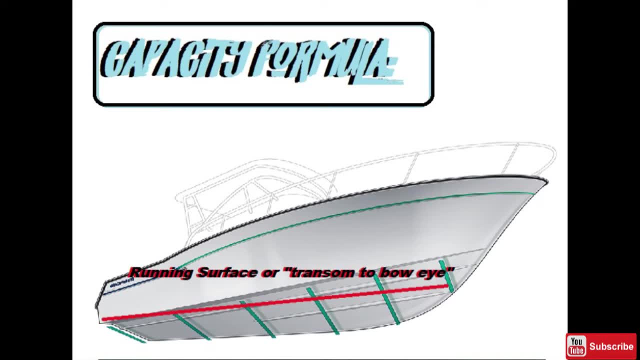 of caution by using the actual running surface transom to bow-eye measurement. the actual running surface- to explain it is simply how much boat is sitting in the water while it's sitting still, hey guys, hopefully i haven't washed yet. okay, it can be confusing when you're comparing all. 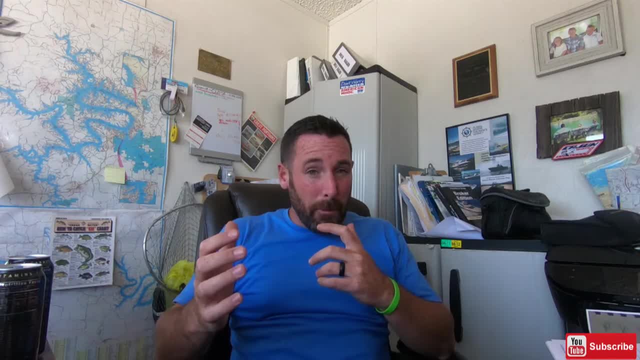 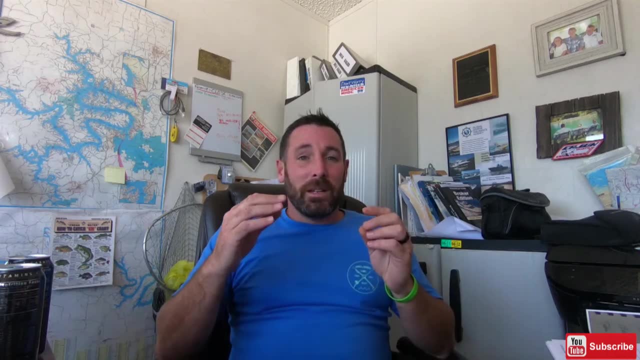 these numbers to the formula, maybe using the boat you own, a boat you're shopping for- with the capacity formula to try to determine a rating or if it's the right boat for you. so because of that, i'm going to use two examples of capacities and boats and kind of show how. 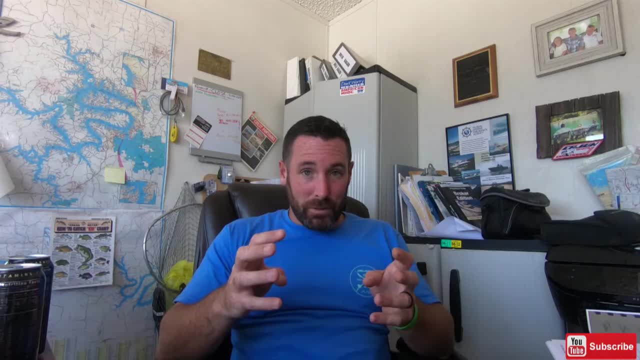 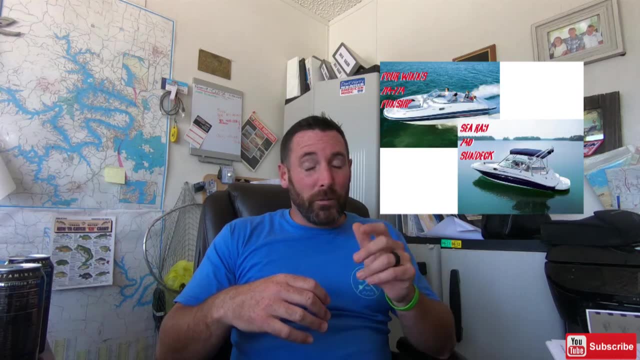 they're different, right, how different companies use different measurements to determine the capacity ratings. so i'm going to use a mid-2000s four winds 224 fun ship- uh, 03-04-05, that was called the 214 fun ship- and a 1999-2008 sea ray 240 sun deck. let's look at these. 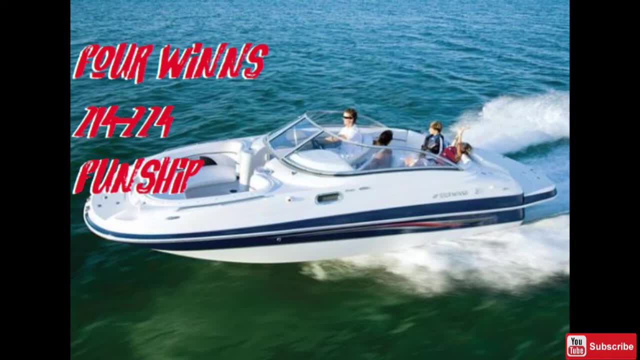 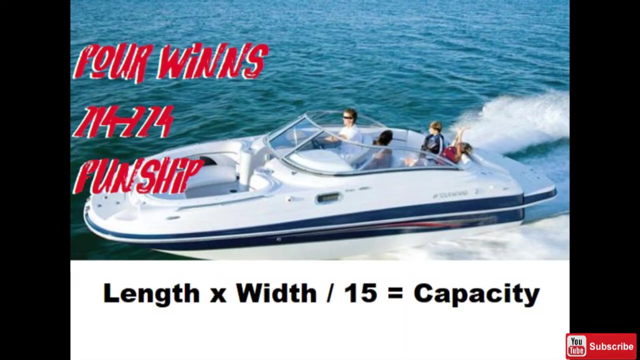 with a four winds 214, 224 fun ship, we have some. this boat's actually rated for 13 people. it has a length overall: 23 and a half feet long. i used a tape measure to get these length without swim platforms: 20 foot 8 inches. the actual running surface of the boat is 19 feet 8 inches. so if 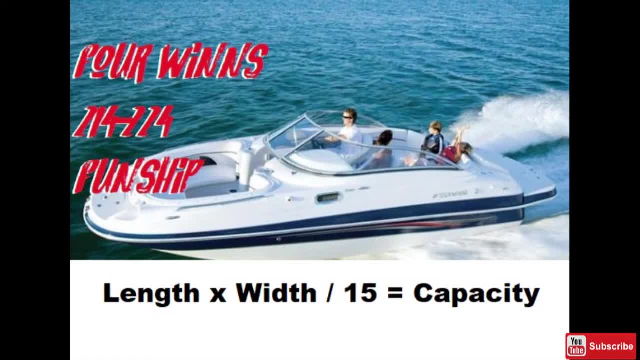 we apply the formula length overall times width divided by 15, that will actually give us a capacity rating of 13 people, so that would be accurate based on length overall. so now let's look at the sea ray 240 sun deck. there's no question that the sea ray 240 sun deck is longer. they're. 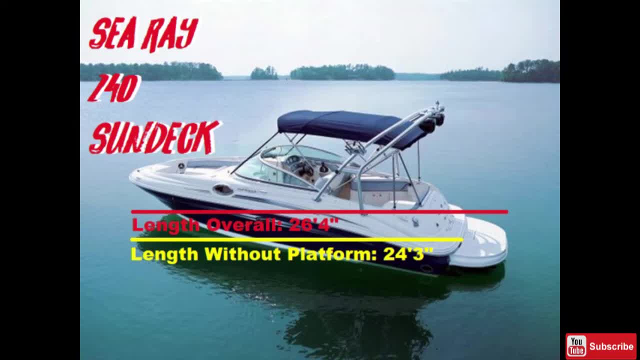 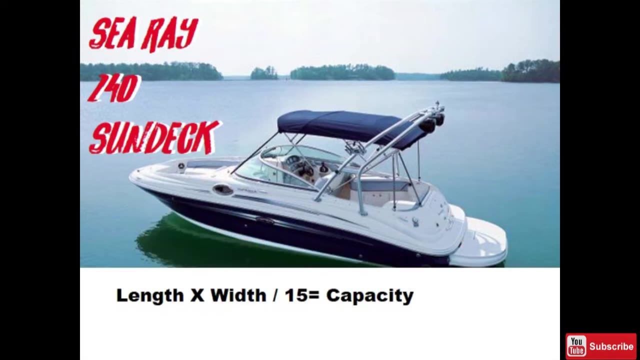 the same width, there's a lot more room in the 240 sun deck. it has a length overall 26 foot 4 inches, length without platform of 24.3 inches and an actual running surface measurement of 22 foot even transom to to Bowie. So using our formula length times width divided by 15, we get a capacity rating of 15. 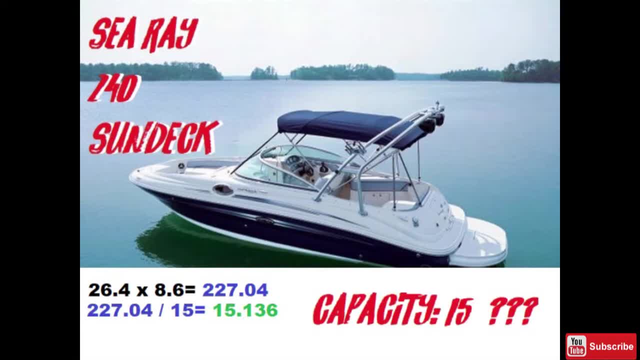 people, That would be right. Winner winner: chicken dinner- right. Sorry, that's wrong. So here's a true example of how companies differ in their measurements. So if you were to apply the length without some platform, you'd still be wrong. But if you apply the running surface, 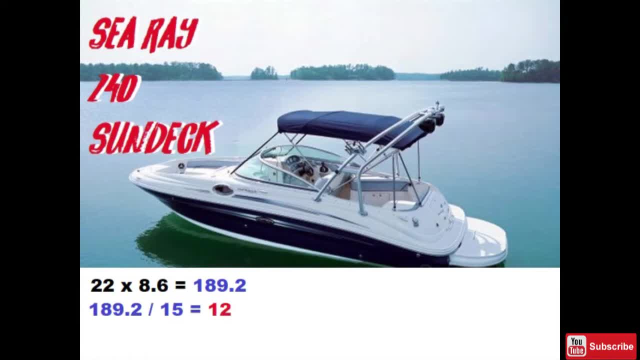 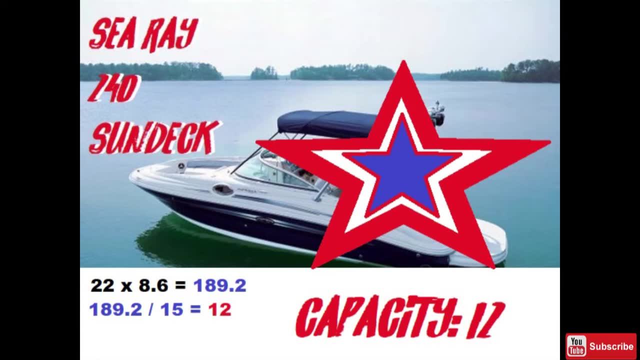 times the width of eight and a half feet wide, do the math, you'll get a capacity rating. Now hopefully you see what I mean by the length overall or the length without platform or the running surface. length of the boat should be more clarified or used to classify the rating. 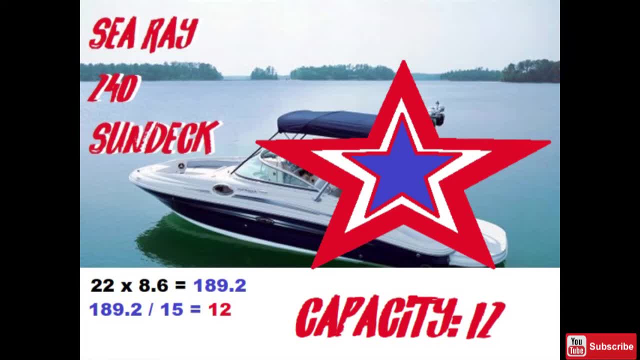 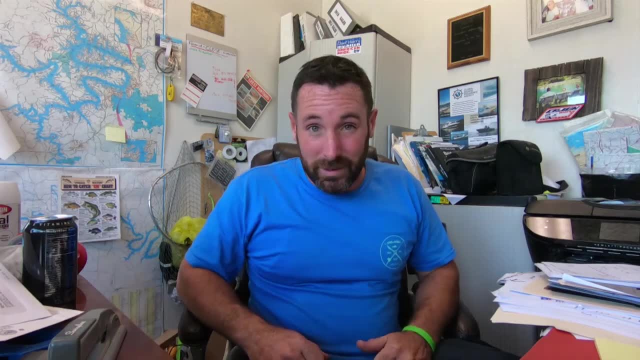 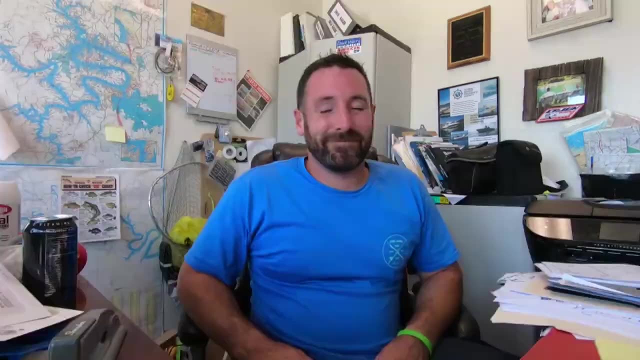 capacities of boats. Well, I hope that helped you. Now for something entirely different. let's talk about yacht certification. Let's talk about what it isn't. That means you can't sink to some bitch. All that means is it can ride in the ocean. None of that's right. 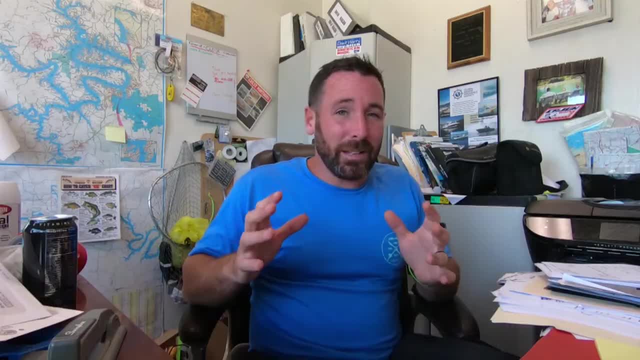 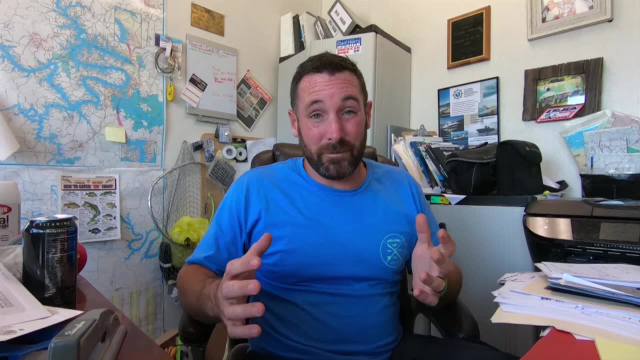 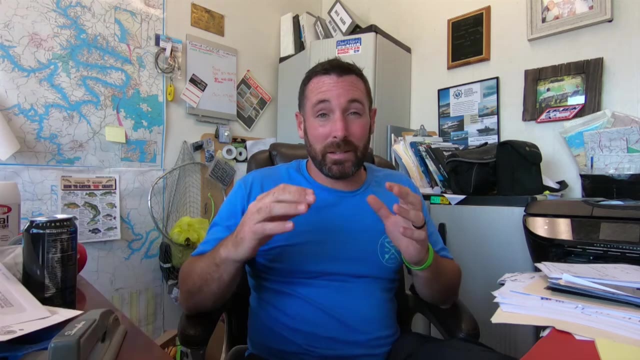 Dammit, will you just leave me alone. As fancy as it sounds, what it really means is well, two things. Number one, it just meets certain criteria. And number two, it's just a label given by the National Marine Manufacturers Association because it meets A, B. 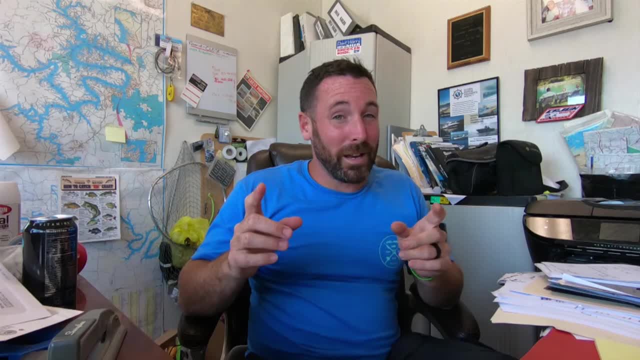 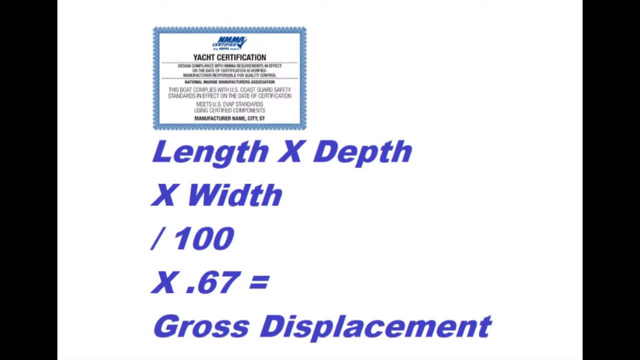 C standards. Let's talk about the mathematical formula that you have to use to determine if a boat's documented or not, though. So to find out whether or not the boat is documentable, this is the formula: Length times depth times width, divided by 100, multiplied by 0.67.. That